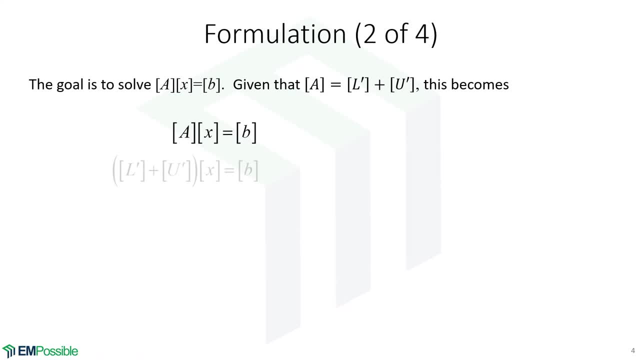 into our equation and see where we are. So we have AX equals B. We split A into L plus U, then we multiply that out, so we have an L times X plus a. U times X equals B. Now we know from experience with triangular matrices- triangular matrices sort of represent: 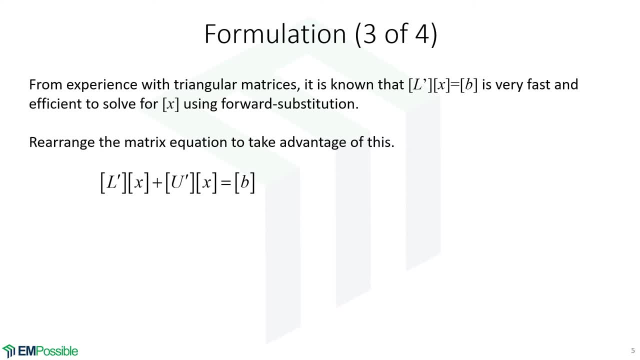 almost solved matrices, So we know they are extremely fast to solve. So if we have an LX times B, where this is a triangular matrix, we know that will be very fast to solve, So let's try to take advantage of that. So here's where we were. We're going to take advantage of that. 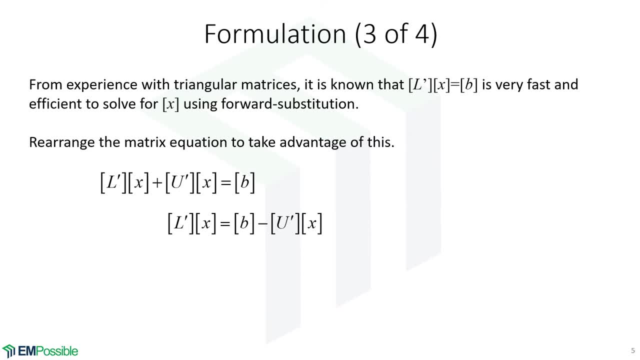 On the previous slide. let's move our U times X over to the right, and that's a U times X. So now we have an L times X equals B minus U times X. Then we'll put parentheses around what was on the right hand side, We'll bring our L over to the other side and this gives us an equation that we 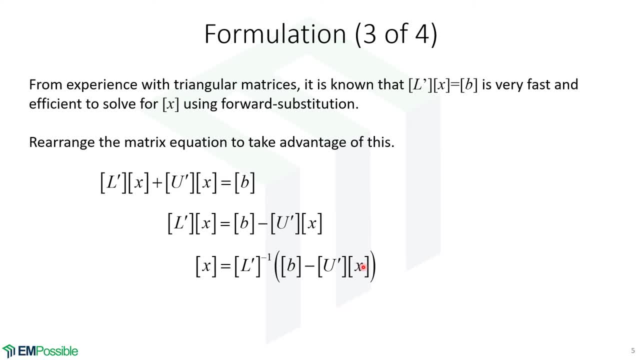 have to solve for X. Here's all multiplication. That's very fast. This is a triangular matrix, meaning it will be very, very fast to solve this problem, And that's really the magic of this method: that we're using triangular matrices that are very fast to solve. 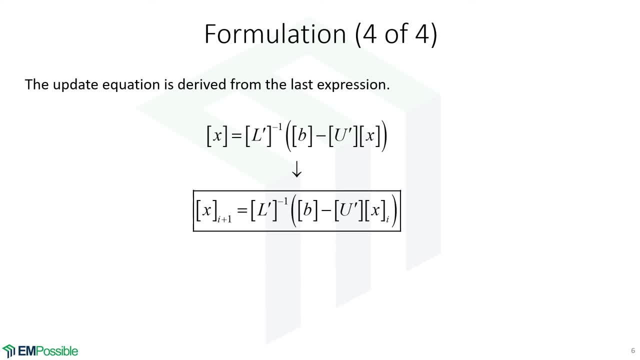 So here's the final form of our update equation. We're just writing this a slightly different way, where we'll put an I subscript on X, meaning this is the X from the current iteration, And we apply this equation To calculate X from the next iteration. And remember, L and U are just, we're just splitting. 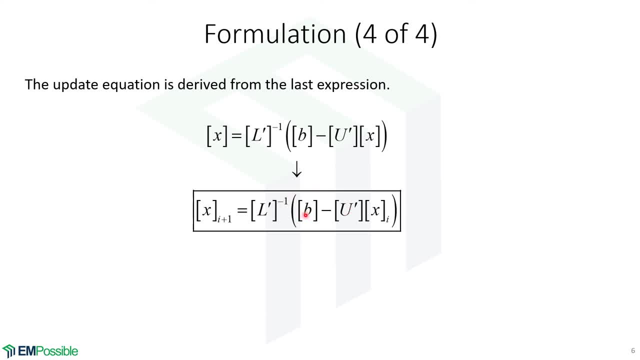 our original A matrix in half So we can put numbers to those. We can put numbers in B and that's a very, very fast thing to iterate And it overcomes the limitation of A having to be a diagonally dominant matrix. From the bottom of my heart, thank you very much for watching this. 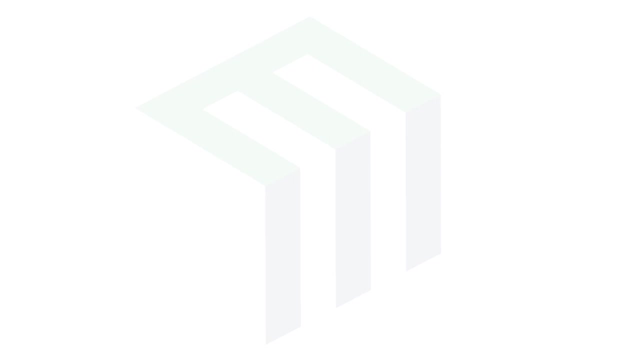 video. I love hearing your stories about how these videos helped you. I also love answering your questions, So please tell me your stories and I'll see you in the next video. Bye. If you like this video, hit the like and subscribe button. I also recommend visiting: